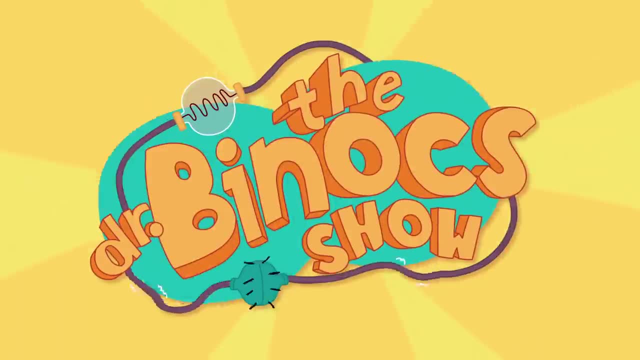 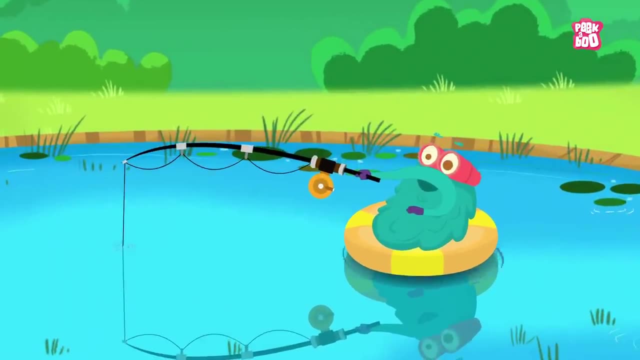 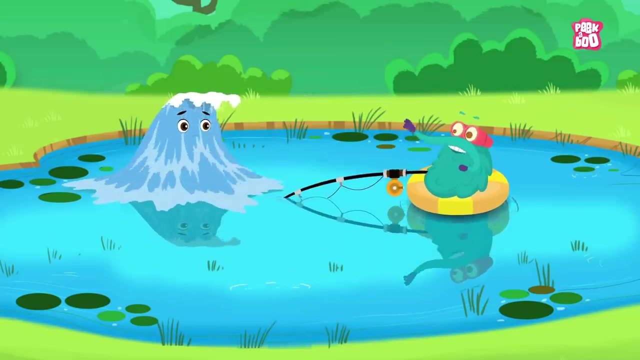 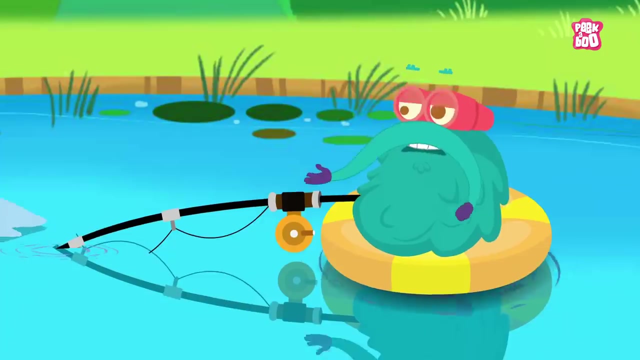 Hey, DrBinox. Hey, who's that? It's me, the pond. Oh, how are you Not good? Humans are dirtying me. Oh, that's sad. They are actually harming our ecosystem. Oh, that reminds me about today's topic. 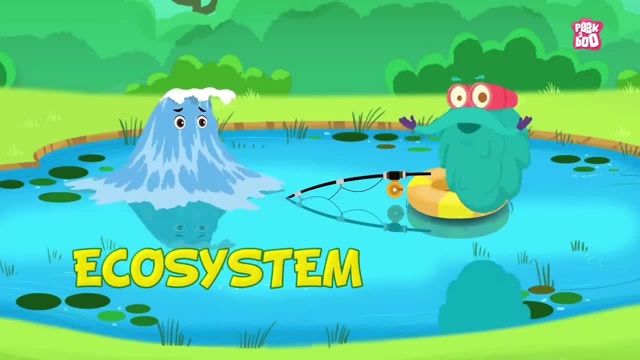 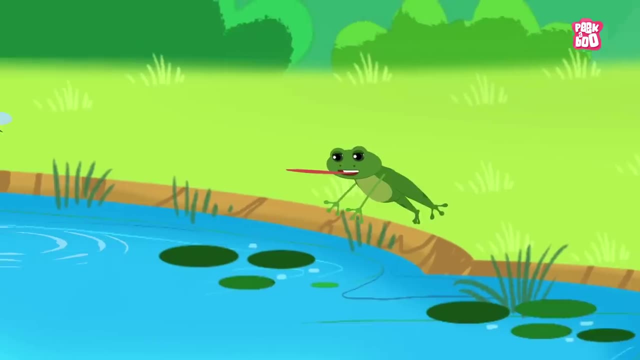 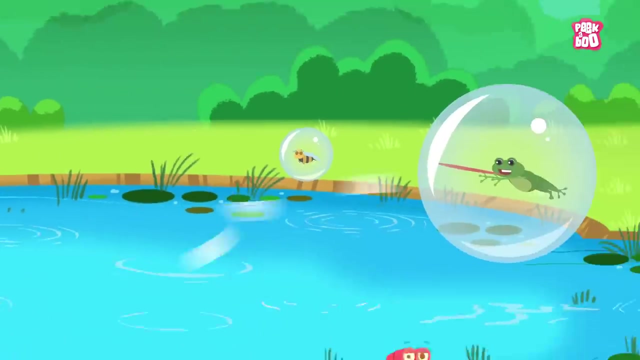 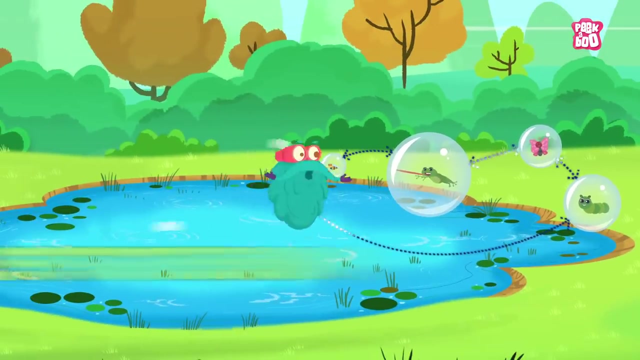 Ecosystem. Come, let me tell you all about it, Zoom in. Ecosystem is a community of living organisms, along with their natural habitat and the non-living components of their environment. This network of living and non-living components in a given area is known as an ecosystem. 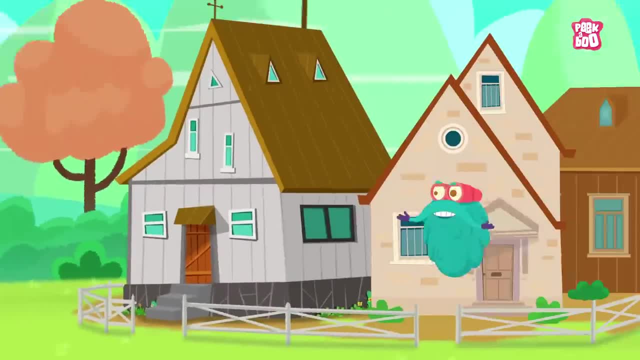 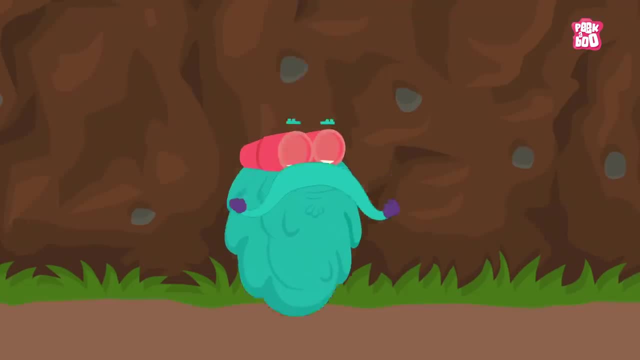 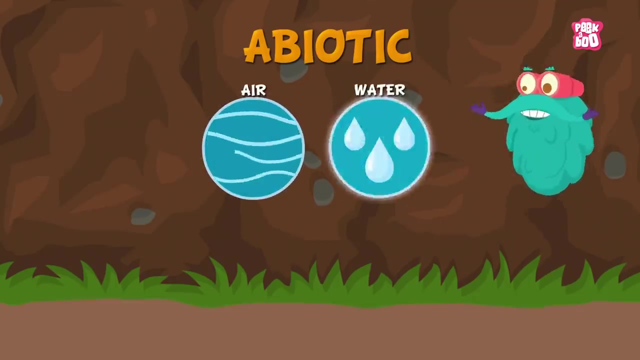 An ecosystem could be a pond, could be your house as well, and some believe that our earth is an ecosystem too. Ecosystem includes two major components: biotic and abiotic components. Abiotic components are the non-living elements of the system, such as air, water, sunlight, nutrients and temperature. 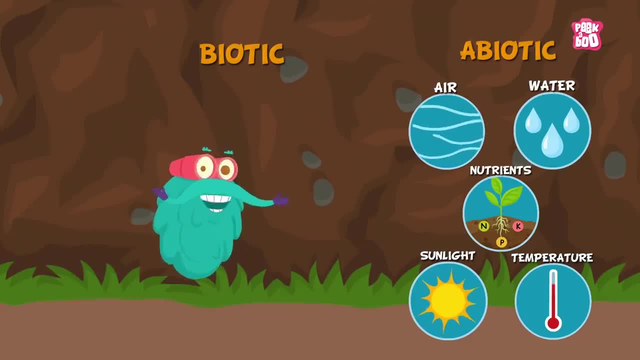 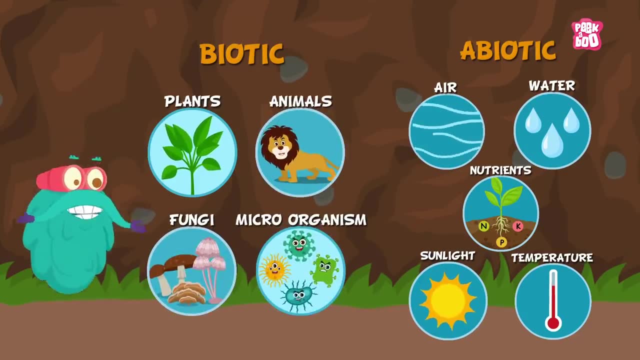 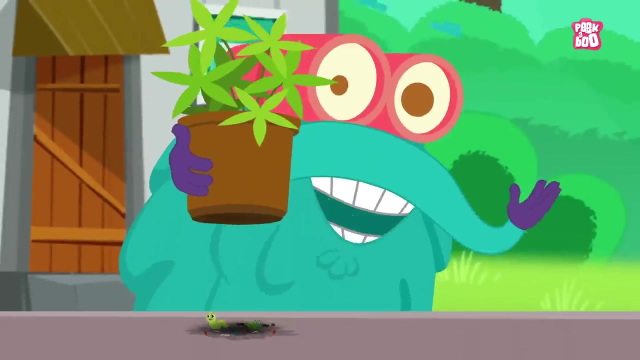 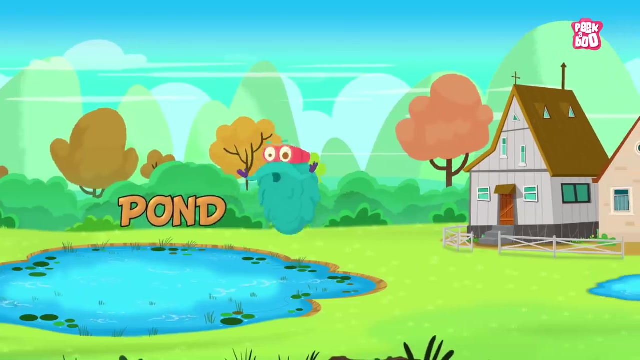 Biotic component are all the living organisms living in the system, like plants, animals, fungi, microorganisms and you. Ecosystems can be of any size: the area under your plant pot, under this rock, a pond, a puddle, the vast ocean, the city you live in. 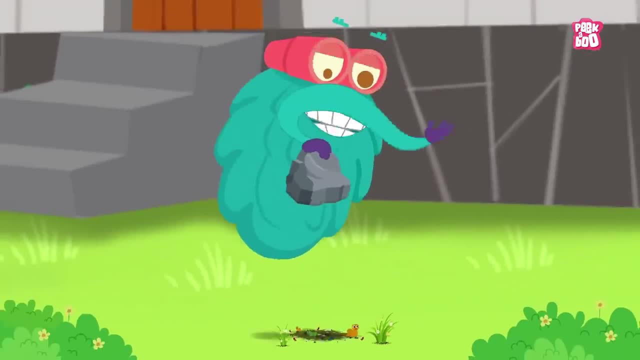 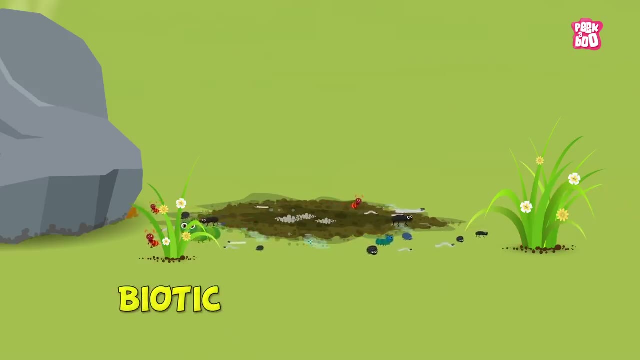 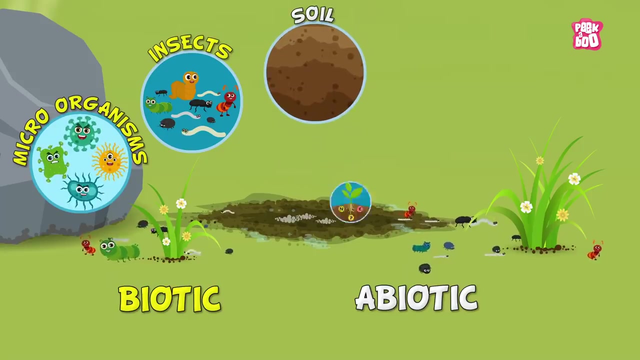 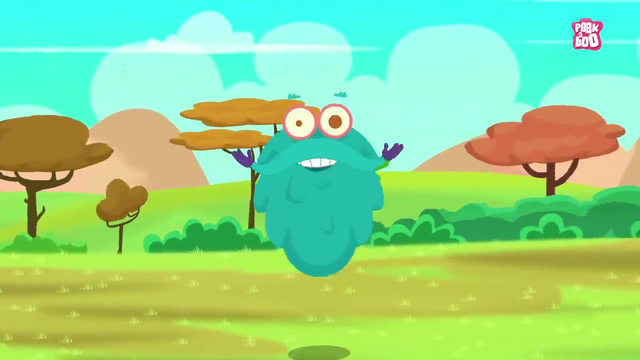 Or your country. Take the area under a rock, for example. In this ecosystem you'll find biotic components, like the microorganisms, insects, and abiotic components like soil, nutrients, air, etc. Now, this is an important piece of information.